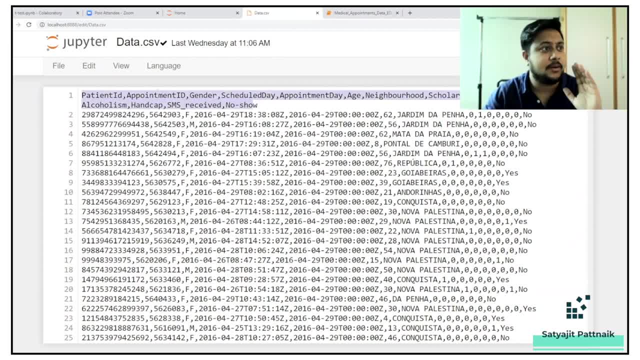 data set looks like. I have different patient ideas, appointment ideas, gender schedule, day appointment, day age, neighborhood, So all these kinds of features I have. And then I have a column called as no show. That means, if it is no, that means the patient has not. 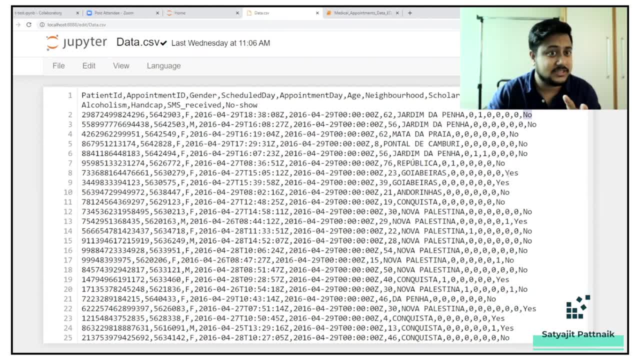 come on the appointment day. Yes means the patient has come, something like that. So, again, this is a classification related use case. If you are building a predictive model, then it's going to be a classification model. But as we are talking about the descriptive part, the descriptive- 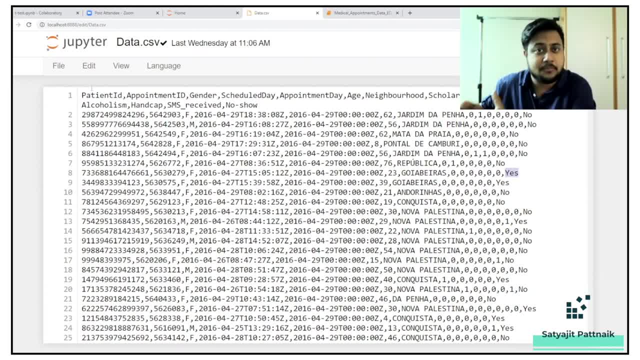 analytics part. so we are not concerned about the predictive model building. We shall be rather concerned about What the data is telling us, what can be the number of features or number of important information which can, which can be extracted from this data set. So let's get started. 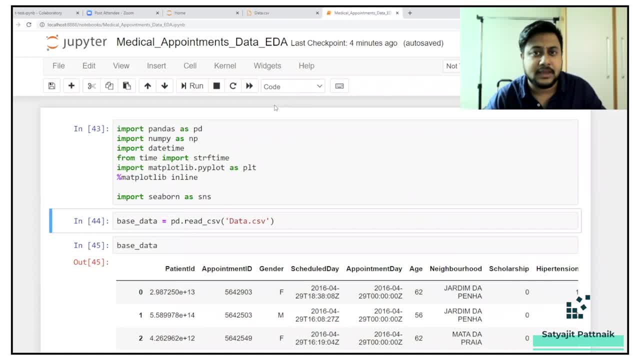 So, as I told you that EDA- if you haven't been through my EDA videos, I also have a dedicated two hours video on EDA. I think that basically covers a lot of topics and that's a very generic video that I have on my channel In case you are looking out for any kind of use case. 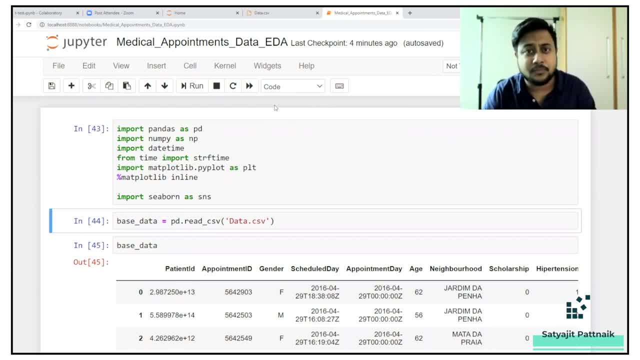 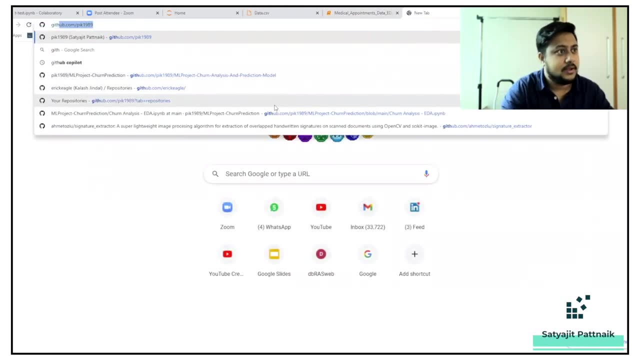 let's say you are working on a business, a banking related or a telecom related use case. You can take ideas from that video and exactly use the same concepts in your data sets. Okay, I'm going to use the same concepts here Now, if you don't know, this is how my data set. 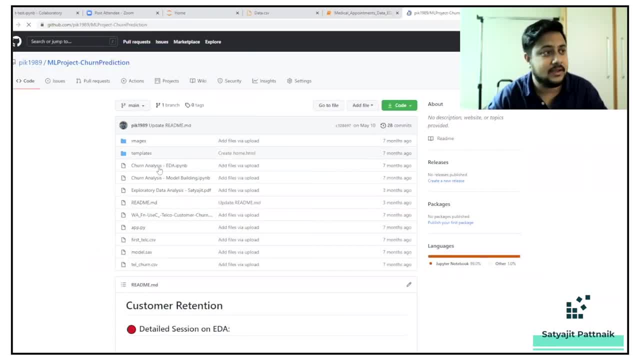 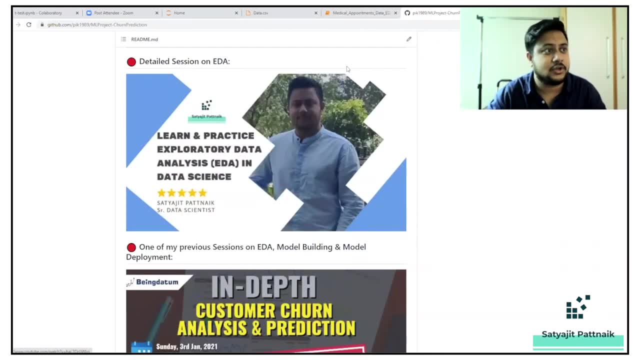 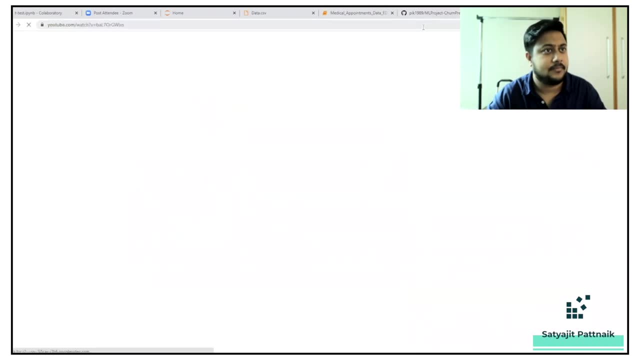 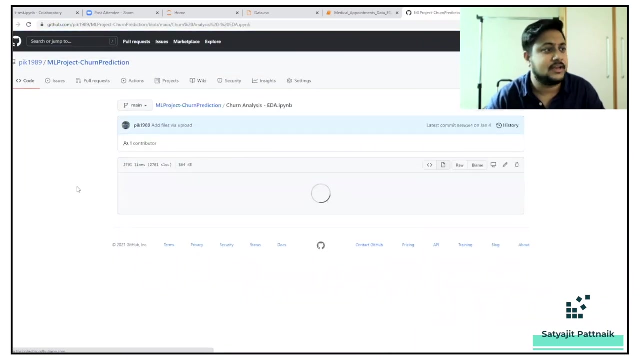 this is how the EDA file looks like in one of my EDA videos. you can see. this video is what I'm talking about: A detailed session on EDA. Okay, I will not be showing you this video, but okay, Uh, it's. it's. anyways, you can just check out this one. and this is the churn analysis EDA file. 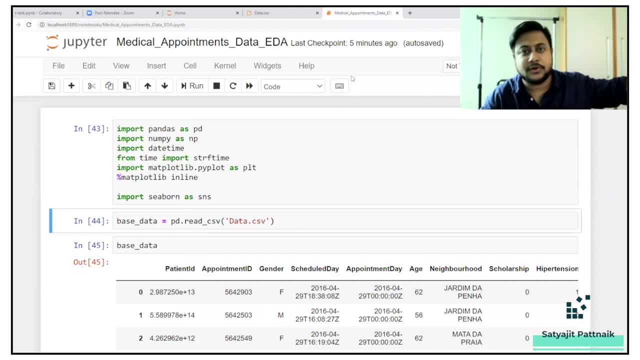 Okay, Let's not talk about that in this video. You can go through that video, check it out. I think that should be okay. Let's get started with the healthcare related use cases. I also have very important Power BI related dashboards as well. 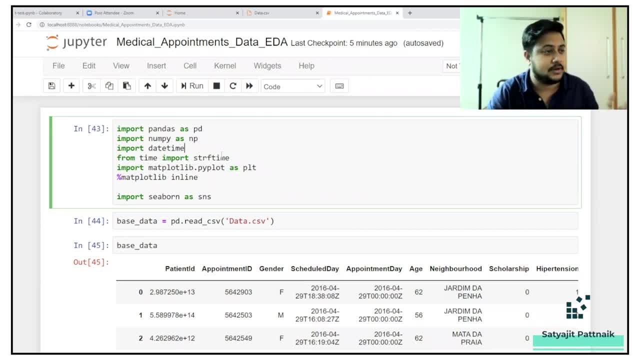 but to get started, let's go ahead and get started. I'm going to show you how to use this. So the power BI, uh, is just for the Python part of the EDA, So here I'm not going to run each and every line of code. 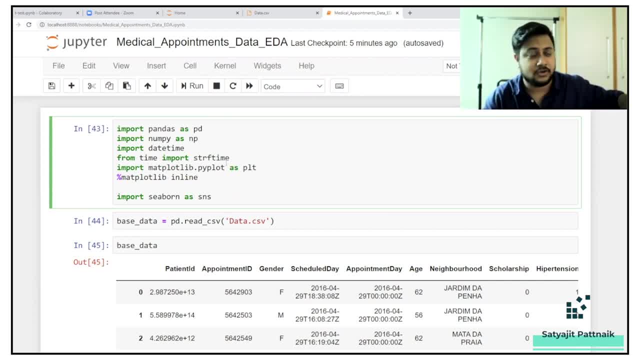 I will leave this to use so that you can practice by yourself, but I will be covering each and every line step by step. Now, when you are doing EDAs, of course, in case of Python, you have to import your libraries. 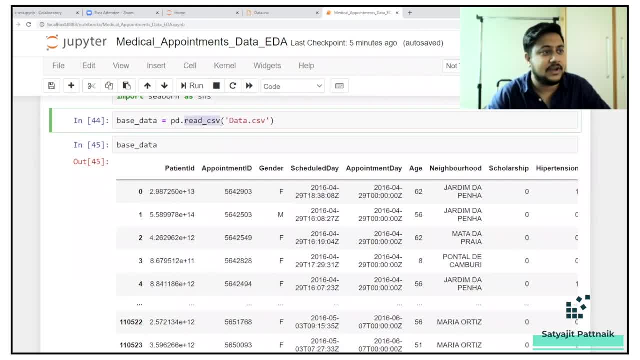 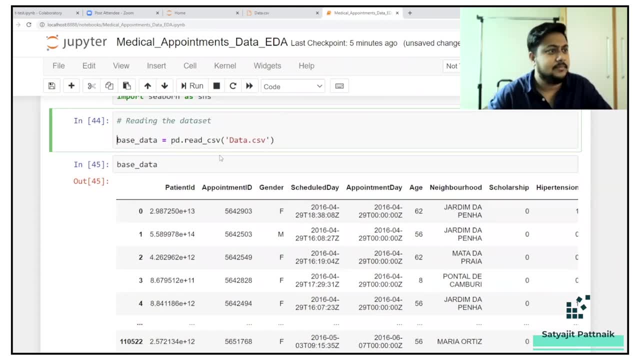 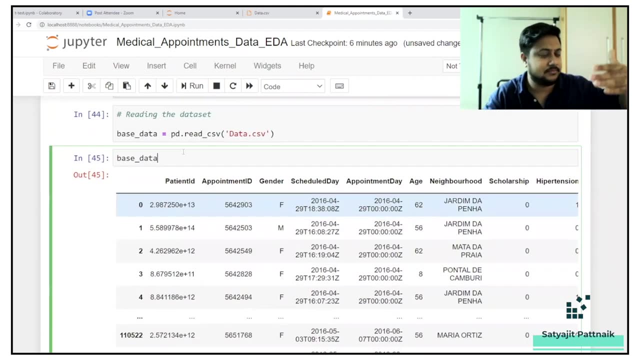 which is pretty much common. And then here I have read the data set. So Reading the dataset, So data set, and then i'm just printing the data set. you can also print using head method or a tell method if you want to see the first five or ten records, something like that patient id and. 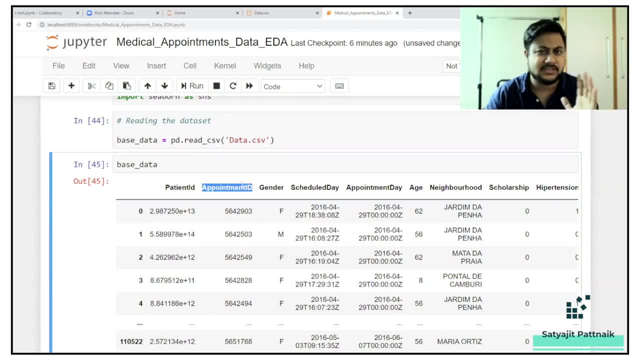 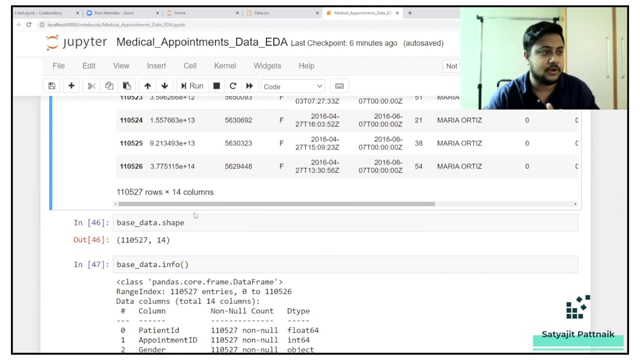 appointment id. these things are the primary case or some kind of auto increment numbers, right? so normally we don't include these in analysis, so we will be discarding this. let's say, your data set has a customer id or some id manager id. ignore it, because analyzing those columns that are auto 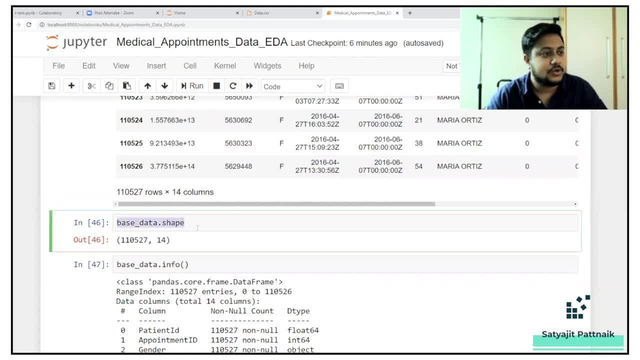 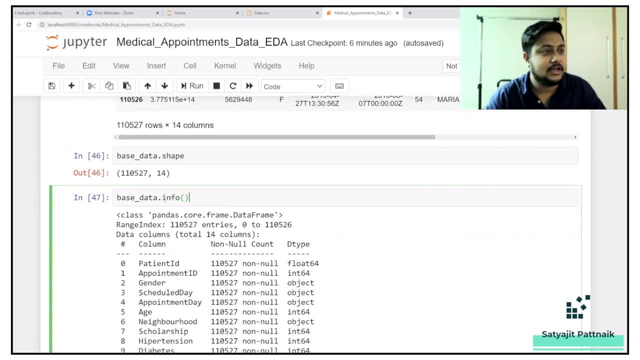 increment columns doesn't make any sense. so data frame dot shape basically tells me how many rows do i have and how many columns do i have. then comes your info method: dot info: see pandas. numpy are one of the most user-friendly libraries, to be very honest. so 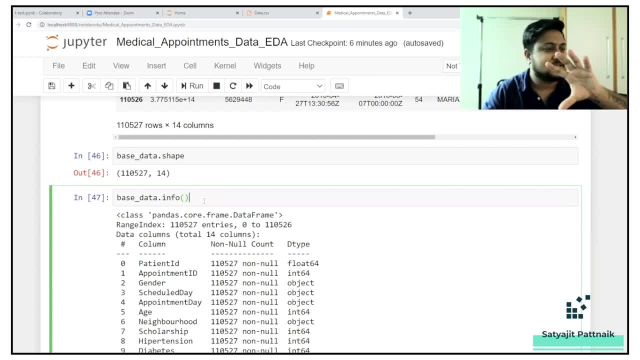 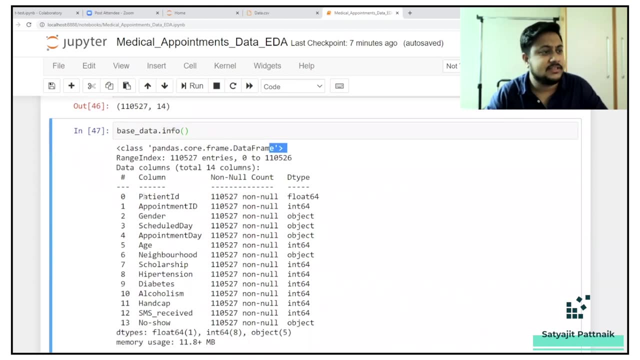 each and every method is so explanatory, it's so self you know. just by knowing the name itself, you will be able to understand what exactly it does. info gives me an information about the data frame. see, i have a data frame. this is the range index. these are my columns, these are my non-null values. now, in this case, i 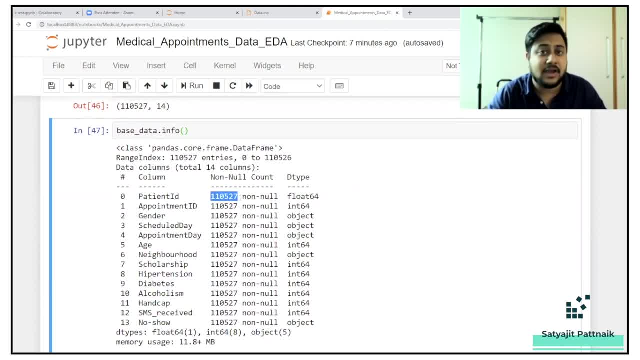 am getting like all the records are having values. that means there is no non-null values. so what does that mean? that means i don't have to do the missing value imputation again. people who are looking out for how to do missing values imputation, i will also come up with. 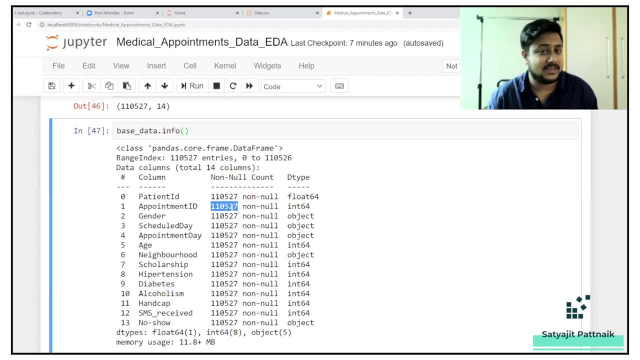 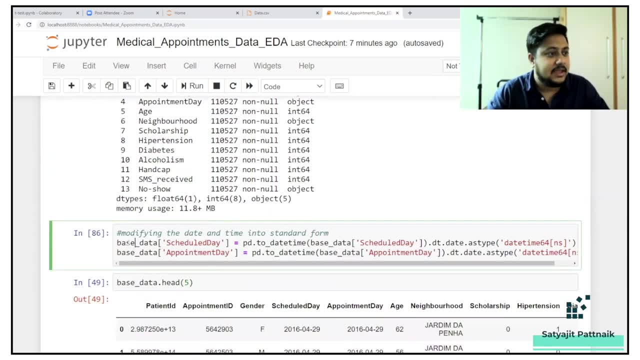 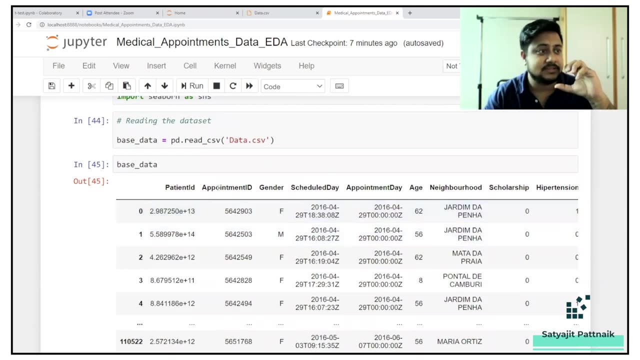 some complex data sets, complex eda case studies, so that you can go through that. but for the time being, let's go ahead with this data set here. what i have done is: you can see so you have heard about something called as derived matrix. right, derived matrix is something like you have a metric from. 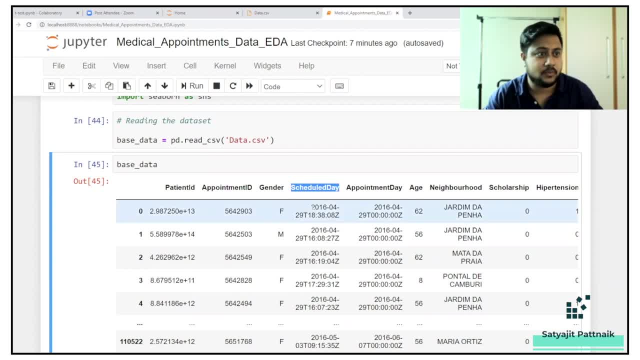 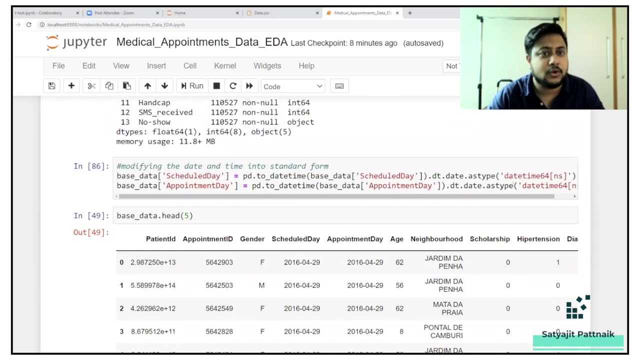 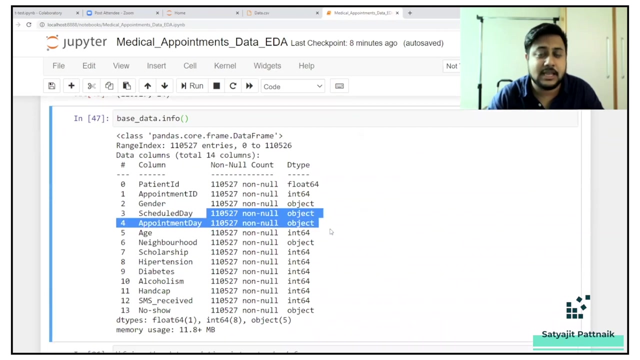 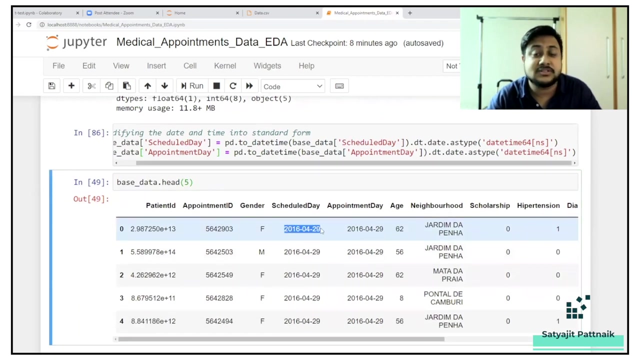 that you are extracting something. so i have scheduled it. so i have scheduled it and i have Low before that it's a object type. you can see it's a object type. i'm converting the object type to a date time, so i'm running this and then i'm running this. you can see that conversion has. 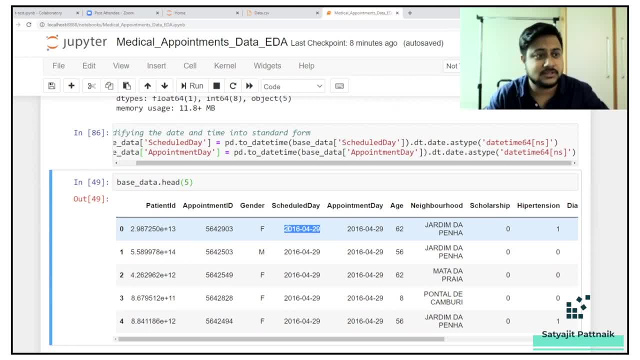 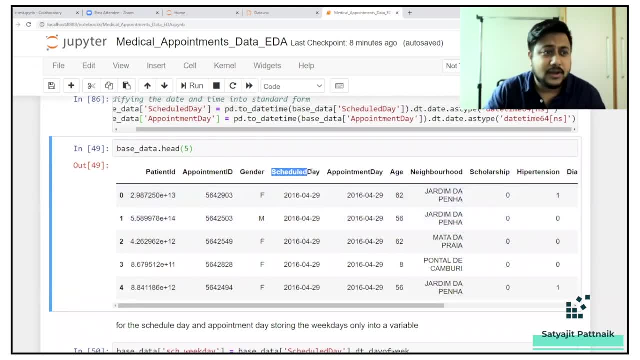 been done right now. We don't need the hour, months and those things. So this has been done. Our next step is, as this is medical data, how can we utilize this method: appointment day and schedule day? So what I thought is, again, you can use your own logic to be very honest, 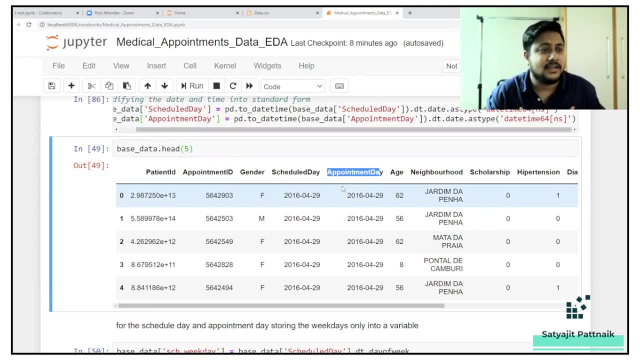 Everything is just trial and error. What I did is I wanted to see: can we get the week number, can we get the day Like: is this a Thursday, Is it a Friday, Is it a weekend, Is it a weekday? 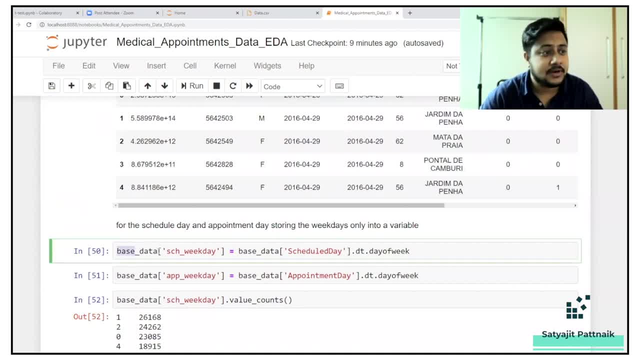 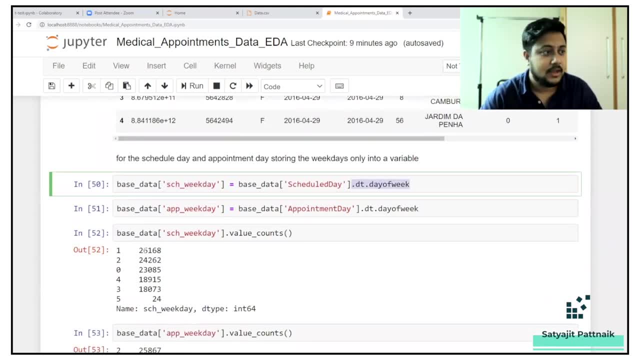 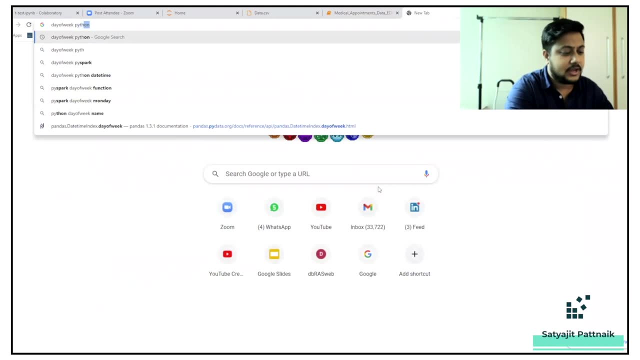 Something like that. So that's the reason I have converted the data into. I have created new columns: SCH weekday. So here I've taken the day of the week You can see here are my day of the weeks. If you are not quite clear what is this method, you can probably check out this one. 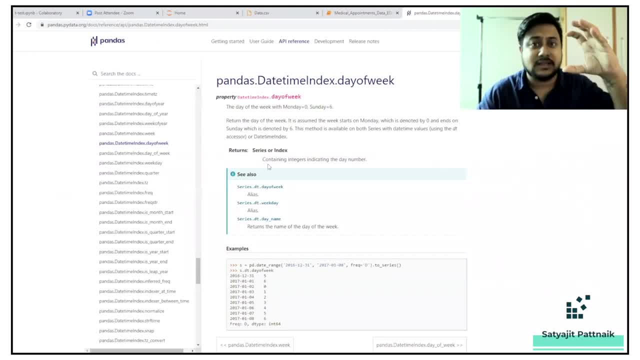 So day of week basically tells you if you pass a date. It will give you which day it is, where your zero means Monday and six means Sunday. That means zero one, two, three, four, five, six, seven days. 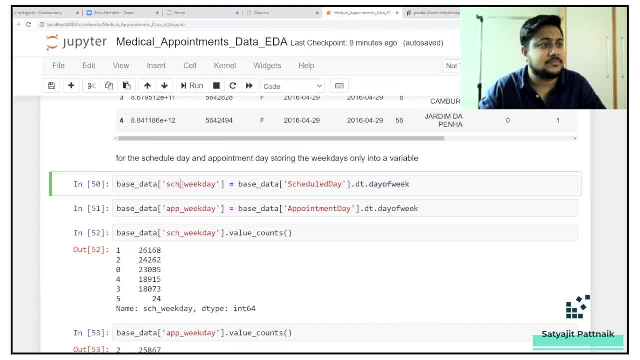 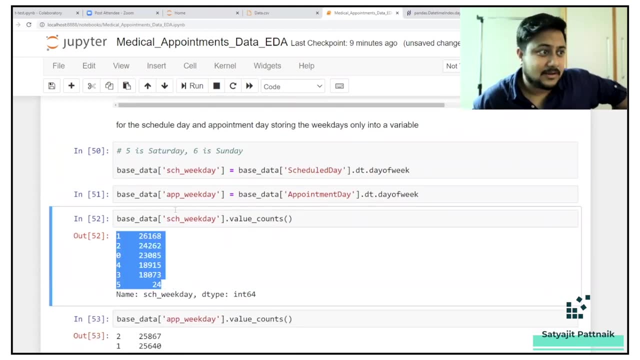 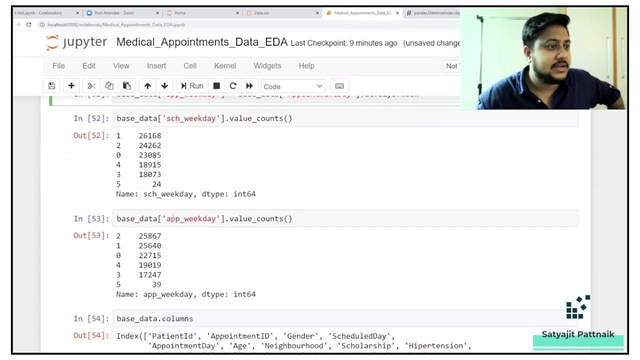 Okay. So it definitely means five is my Saturday, Five is Saturday and six is Sunday. Okay, To be okay. Now you can see these are the days. that means I don't have anything for six. That means there is no scheduled day for Sunday for application day. 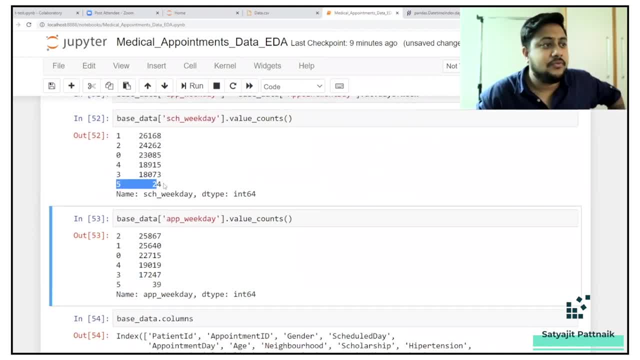 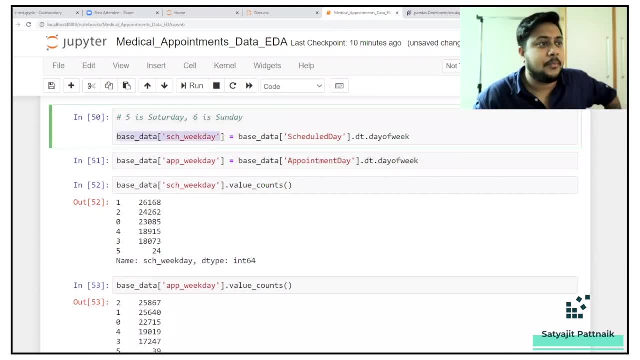 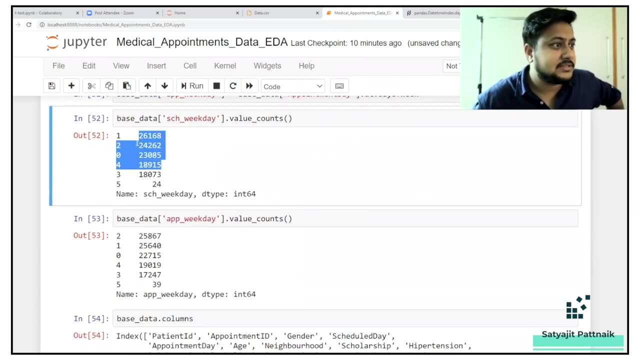 Sorry for appointment day. Also, there is nothing for Sunday, only for Saturdays we have. So what do we infer from this? We infer that most of the appointments and the scheduling is happened between the weekdays, not in the weekend, Again in the weekdays. if you want to analyze, you can see. this is how the data looks like. 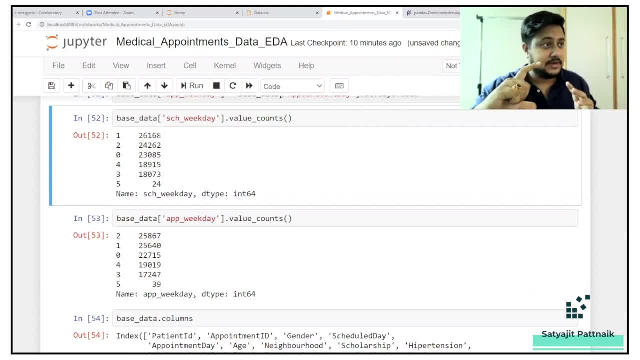 You can also plot a bar graph to understand for Monday how much Forty-one Tuesday you can see for Monday, Tuesday and Wednesday. I can see the large number of values. maximum for Tuesdays right And again during the weekend is going to come on Thursdays and Fridays. 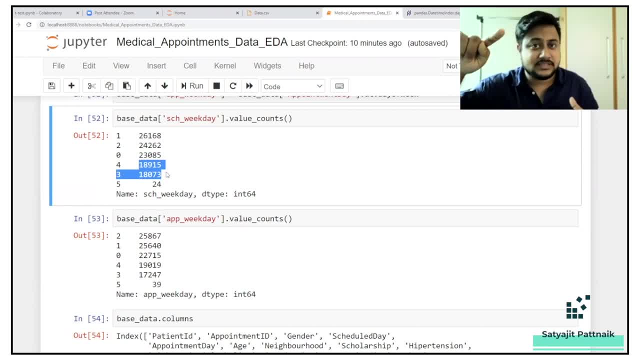 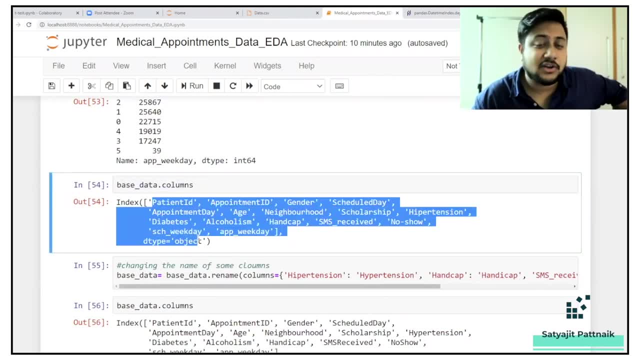 The numbers are decreasing. That means there is a trend of increase during Mondays to Wednesday, and then it is decreasing. as simple as that. Then I'm doing the dot columns, where I'm seeing the columns, And then here I'm just changing some names. 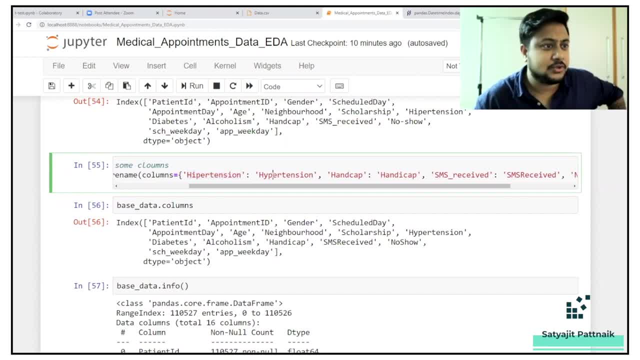 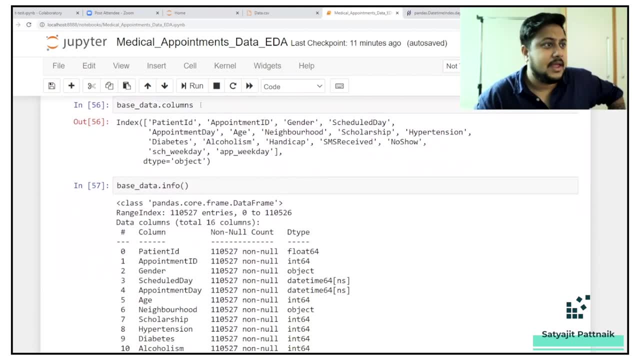 There are Some spelling mistakes. I'm just changing hypertension to hypertension and cap to handicap, so that we can read it easily. right? No show to no show, something like that. And then again I'm printing the columns and again I'm doing the information. 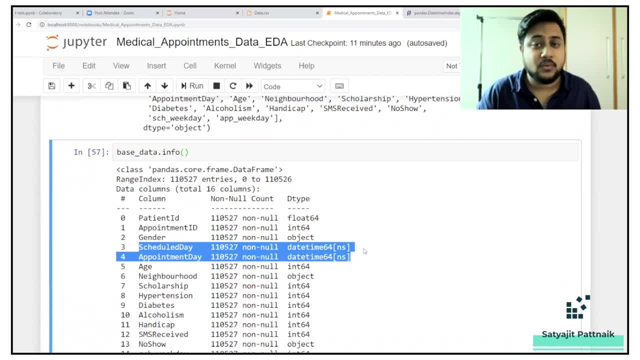 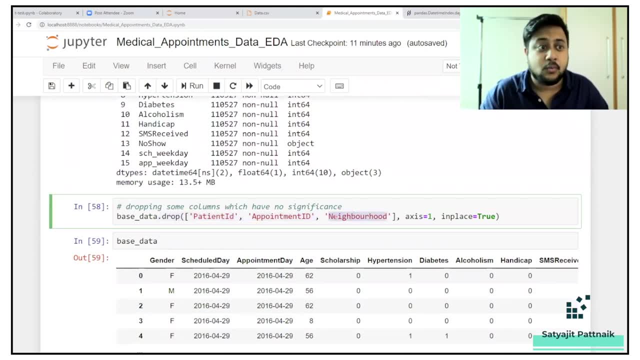 So here you can see: previously it was object type, Now we have date time. Okay, Then I'm dropping the patient ID, appointment ID and neighborhood. Now why neighborhood? When I started doing it I actually dropped these two Columns and then I ran some methods and then I came back and then dropped neighborhood. 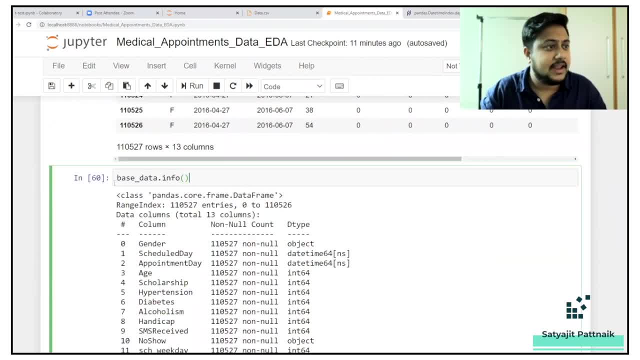 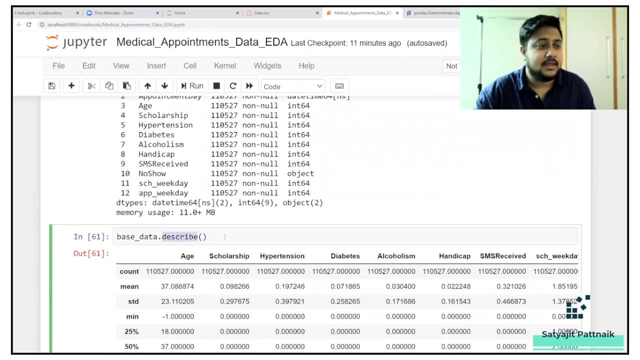 I'll talk about neighborhood later on And then I have again done the information. You can just ignore doing all these things again and again. describe method, As we already know that it explains the statistical information right. As simple as a block spot, a box plot, box plot and a Vista plot gives you five measures right. 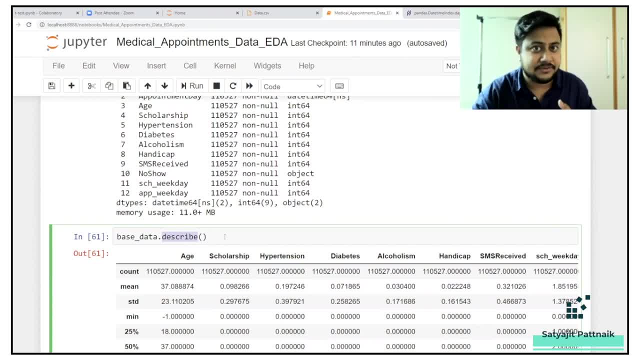 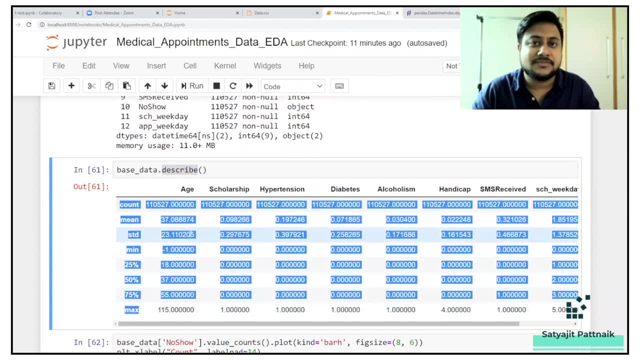 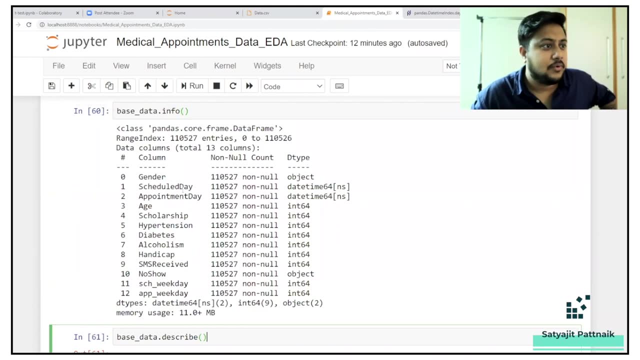 Minimum, maximum, median, 25% and 75%. Similarly, your dot describe methods also gives you the output and it only gives you outputs for your numerical values. It will not work for categorical values. You can see for categorical and for date time values. it's not there right here. 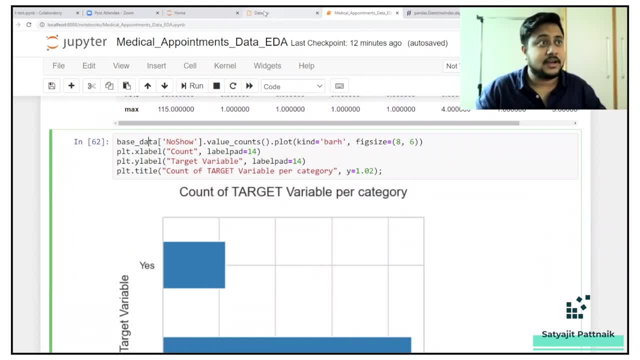 Next step is I'm plotting my target variable. So what is my target variable? My target variable is no show, So I'm trying to plot it so that I can see what is the distribution between the different variables that we have. So, for yes, we have this much and for no, we have this much. 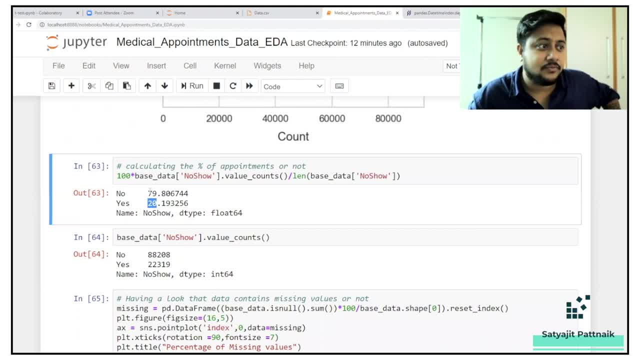 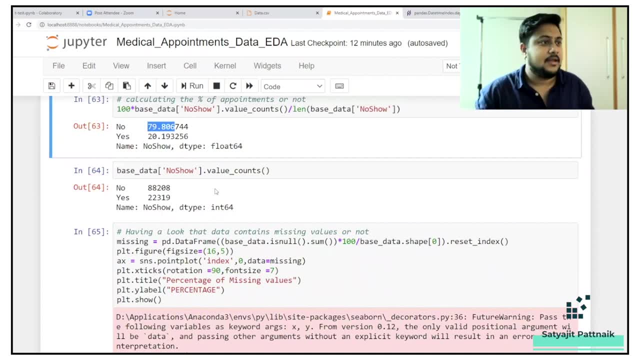 What do we infer So? for yes, we have 20% and for no, we have almost 80%. So the inference is that it's a highly imbalanced data right And our focus is to analyze the minority class. Okay, 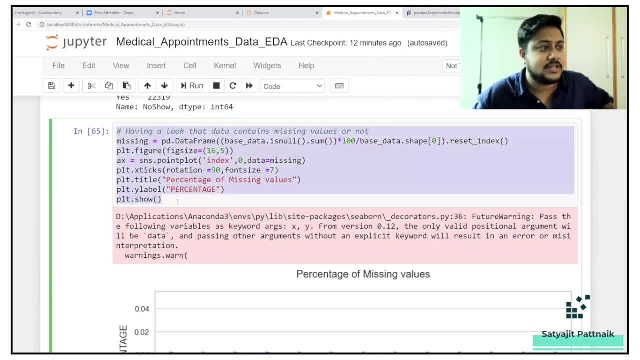 So here, having a look at the data. So this is one of the quotes that I have written for finding the percentage of missing values. You Can, as it is, copy the code as it is, because I have done the same from my previous notebook. just copy. 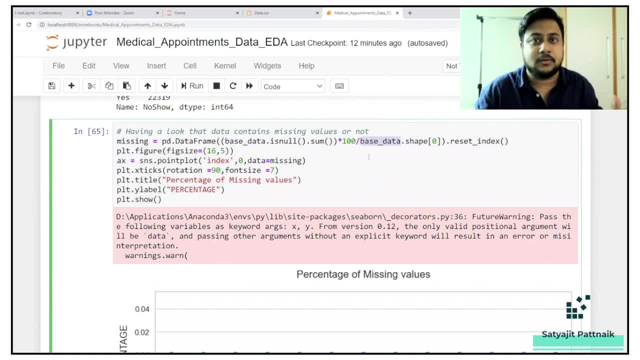 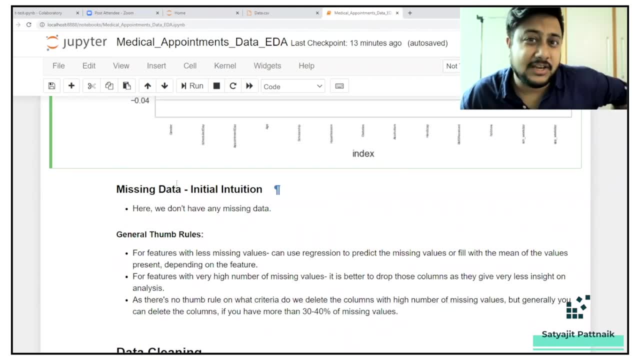 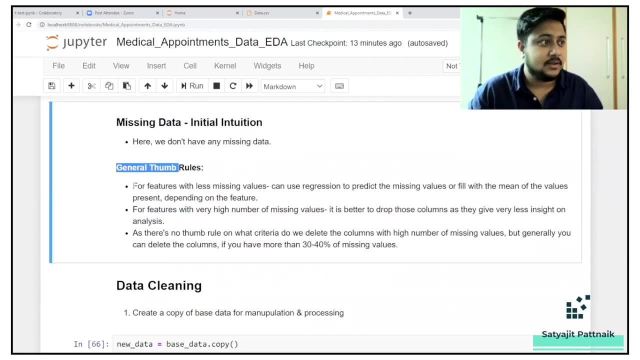 paste it and just change your data frame name here and here, Simple, Okay. Then comes your missing value in missing value data, like initial intuition. What is the initial intuition from this data? here We don't have any missing data, but the general thumb rules are: if you have some missing values, you have to. 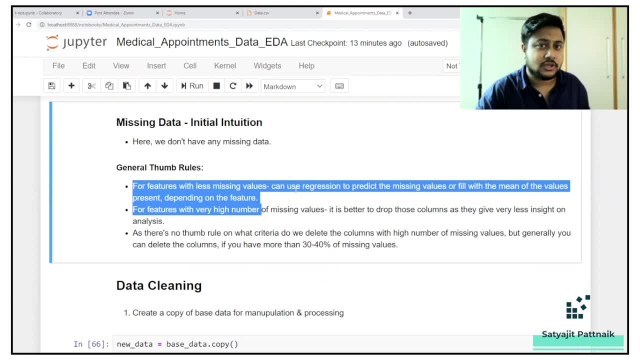 impute using a regression technique or mean value. We will come up with some use cases where you can actually see how I'm using regression to do prediction. Okay, Let's keep that for another video, Then it's not a part of this scope. 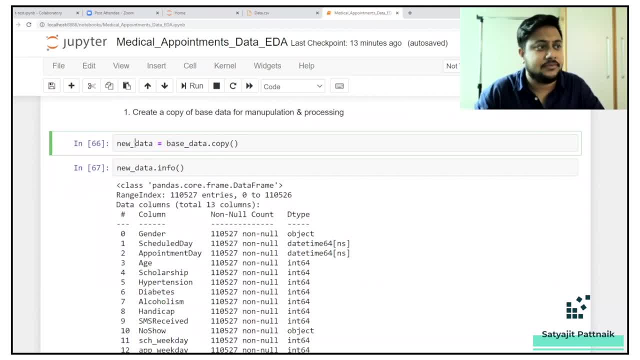 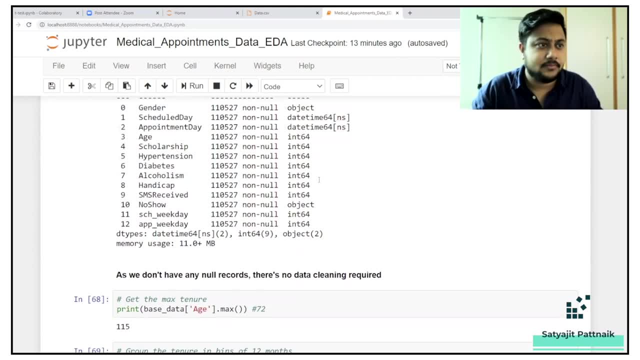 Then comes your data cleaning, where I'm just copy pasting my data frame to create a new data from copy And then, as we don't have any null values, there is no data cleaning required. Very simple use case, but definitely people who are looking out for writing something in the resume, as you can. 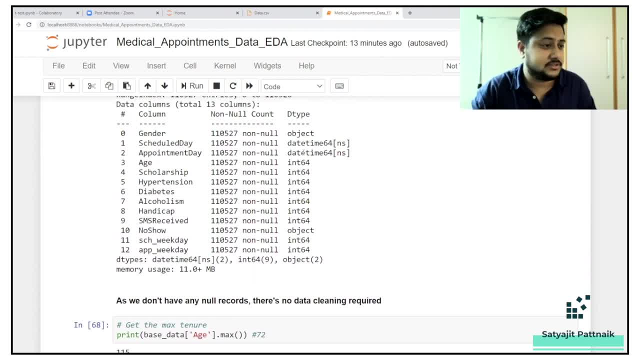 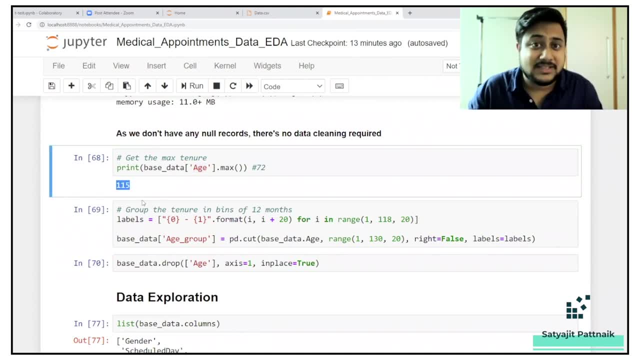 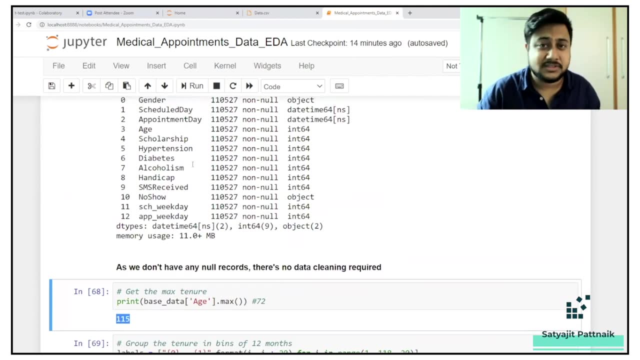 Use this and you can write down in your resumes, especially freshers. Okay, Here I have age column. Now, what is the maximum age that I have? 115.. What is the minimum age that I have? Of course, I haven't printed it out, but I know that the minimum age is around 11 or 10.. 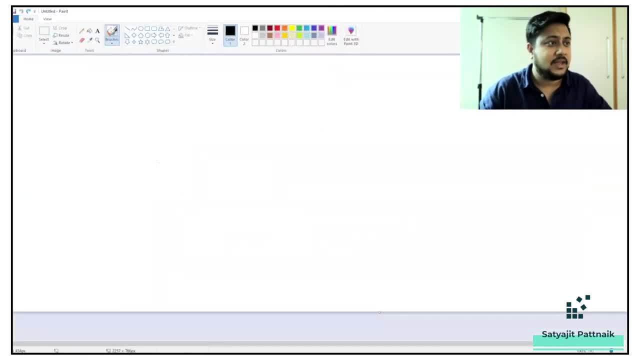 Okay, Now can we plot the age graph, Like, if I start plotting it, let's say I am plotting a bar graph, So it looks like this, right, Something like this, And it will have From 10 till 115.. 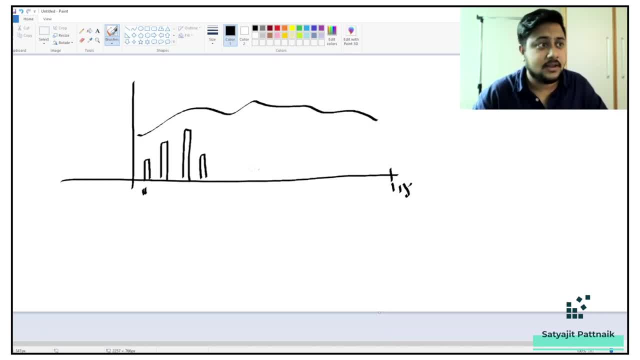 So how clumsy it will be, Just imagine that. So what I have done is, from this numerical data I'm converting into bins so that I can have from age one to 10, from 11 to 20,, something like that, And 60 plus something like that. 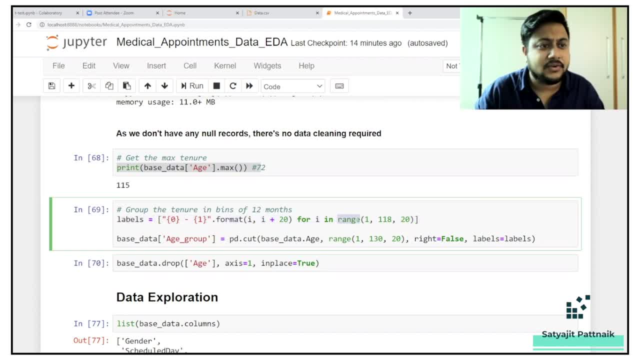 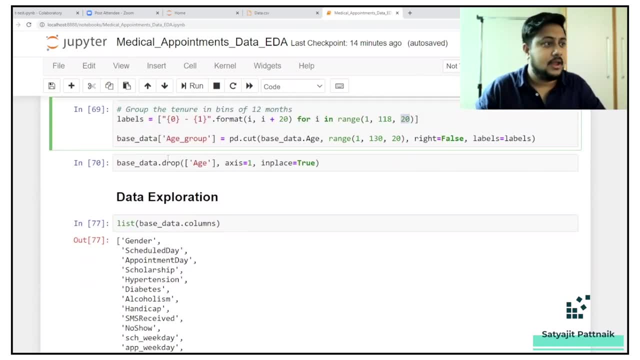 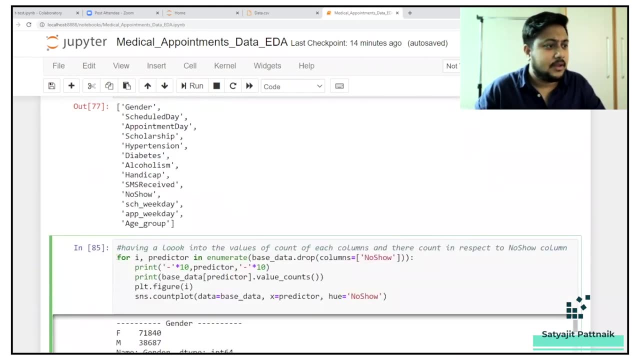 So here I have created bins for I in range of one to one 18, within a bin of 20, that means one to 21,, 21 to 41, something like that. Now, here I have done it, and then exploration starts. you can see this piece of code here for I, in predictor, in enumerate: 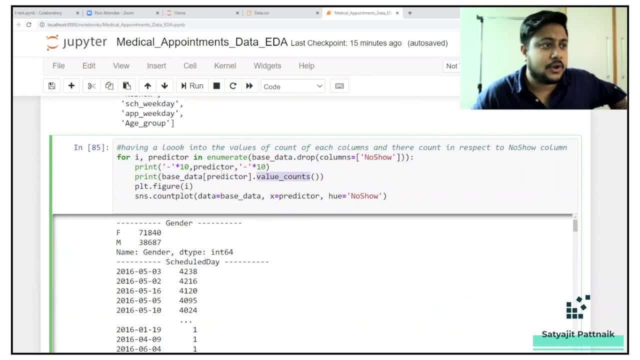 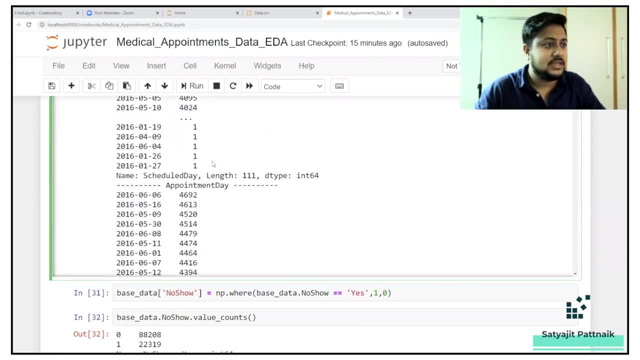 So what I'm doing here is I'm taking a value counts for each predictor. What is each predictor? Each predictor is by each column of the data frame You can see. it gives you the split of data: appointment date: zeros and one. scholarship: zeros and ones. 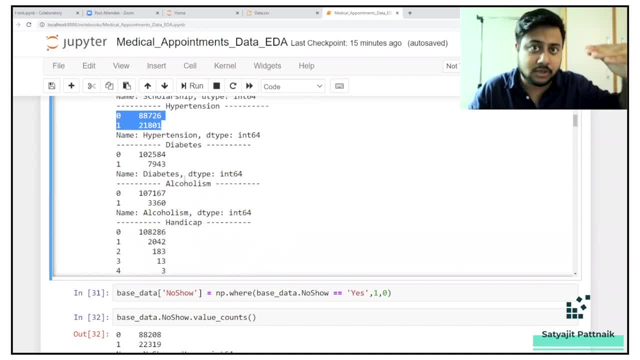 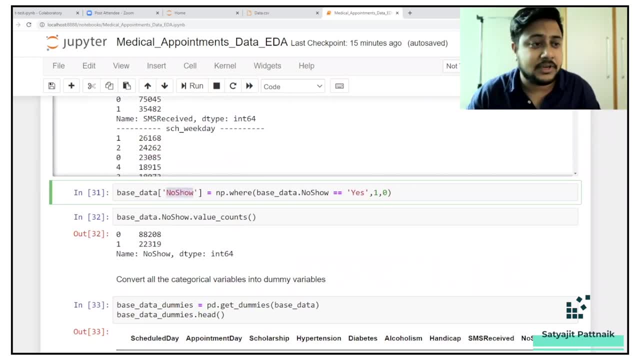 So it gives you a complete idea, Okay, About how the distribution of the data is. Then what I have done is I have converted my target variable to ones and zeros, So I have just replaced it with zeros and ones, And now we have same same data: 80% and 20%. 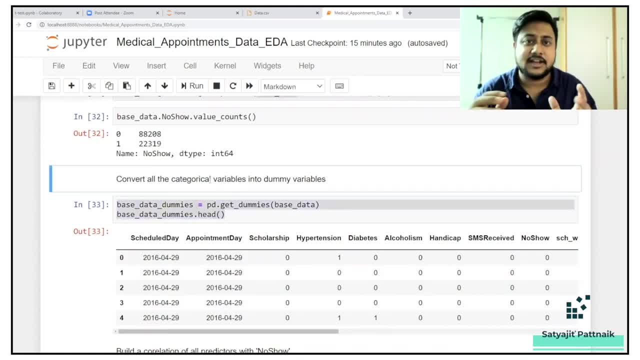 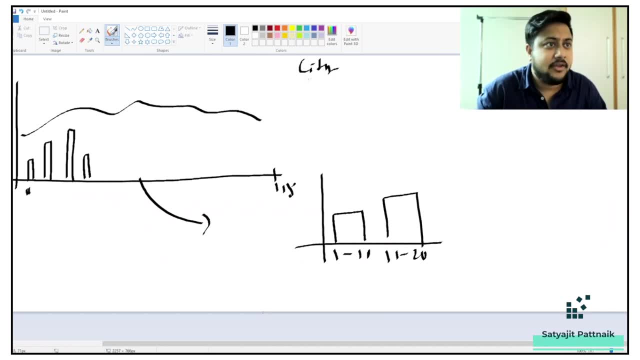 Then I'm converting the data into get dummies. Now, get them is what is get them is. everybody knows about one hot encoding right. So let's say you have some data like this: You have, You have city, you have Mumbai, Kolkata, Hyderabad. can we directly in market as zero one, two? 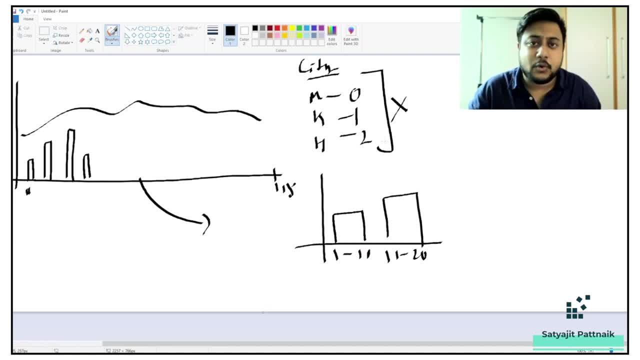 No, this is a wrong way of doing it. Label encoding doesn't work for independent variables, It only works for dependent variables, only works for target variables. If we do this, what happens is our machine learning algorithms or our statistical models give high priority to Hyderabad. 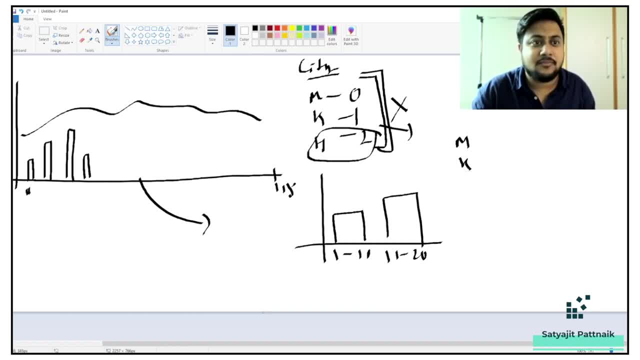 So this is how it works. So a good way of doing is: let's say: I have Mumbai, I have city Kolkata, Hyderabad, Mumbai city. what I will do is I'll create three columns: city underscore Mumbai, city underscore Kolkata and city underscore Hyderabad. here one zero, zero, zero. one zero, zero, zero, zero, one one zero zero. 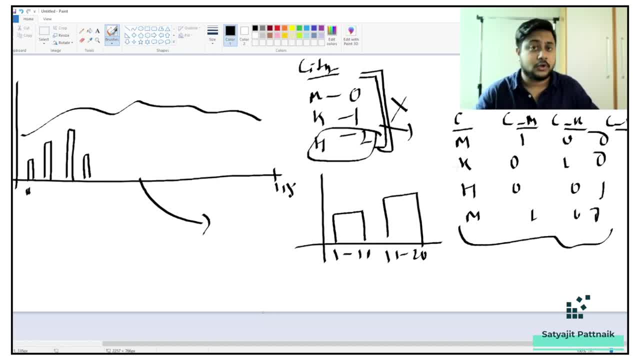 So we are converting data into zeros and ones. If you're not quite clear about the different types of encoding, I also have a video for that in my channel, probably, If I remember. I will put that in the eye section so that you can view it. 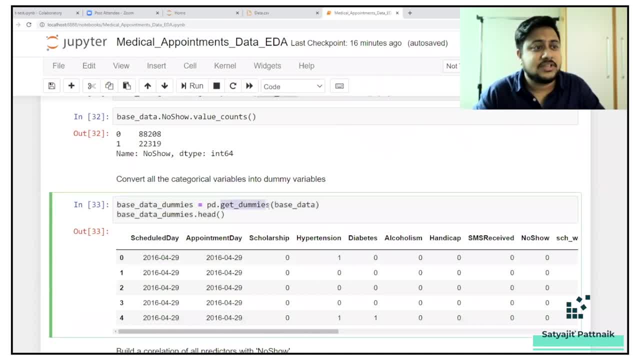 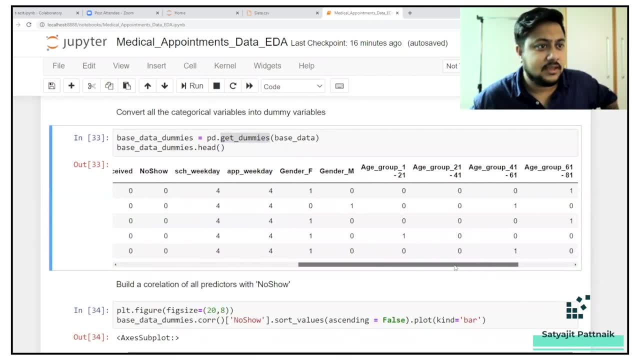 Right away. So I'm using get dummies, which is a different way of doing like one hot encoding. OK, you can see here, if I just see: gender underscore F. gender underscore M: age group one. age group two. age group three: 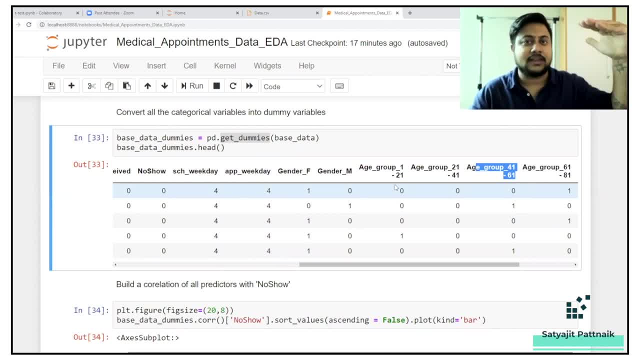 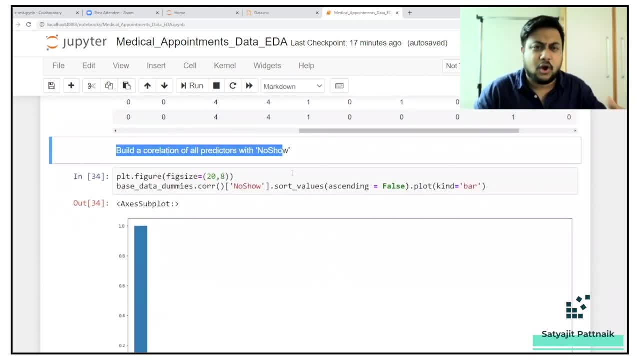 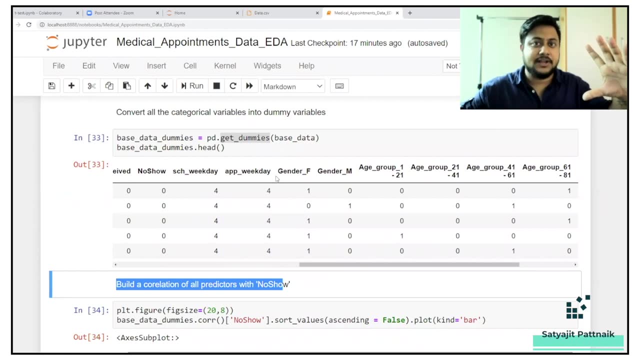 So for each, for each categorical variable, we are creating new columns, OK, and then we will be dropping the old columns. I mean automatically in get dummies, it drops. drops the original columns. So let's say you have gender, it creates gender M, gender F: it drops the gender column. 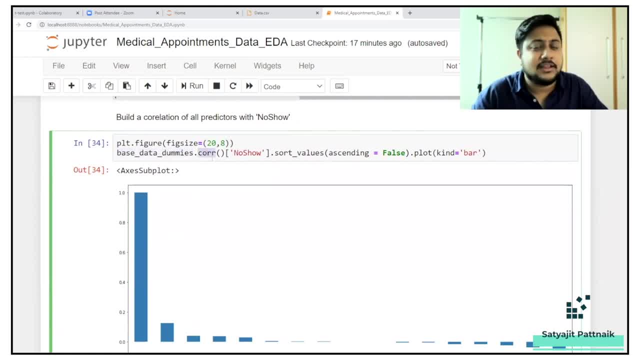 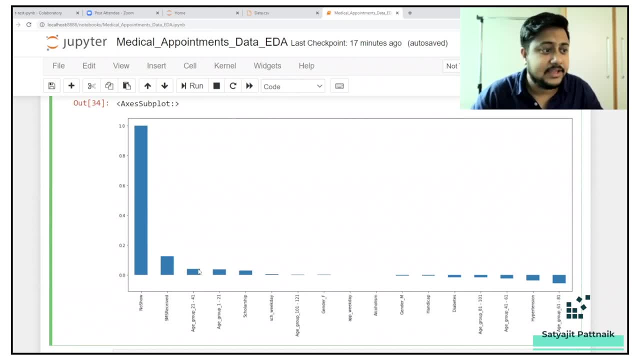 OK, and then I'm just creating the correlation function and I'm plotting it So you can see SMS received is highly correlated. Age group 21,: 41 is highly correlated. Like as compared to other columns, it is highly correlated. Of course, the correlation value is very less. 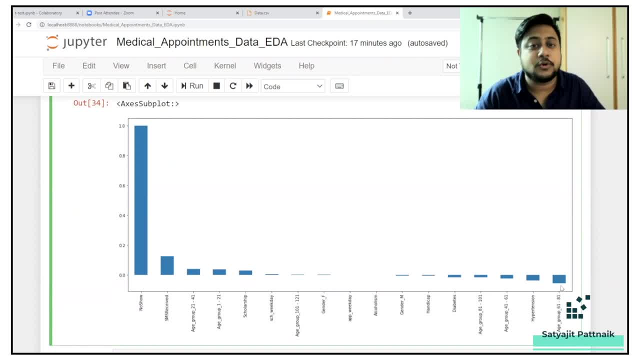 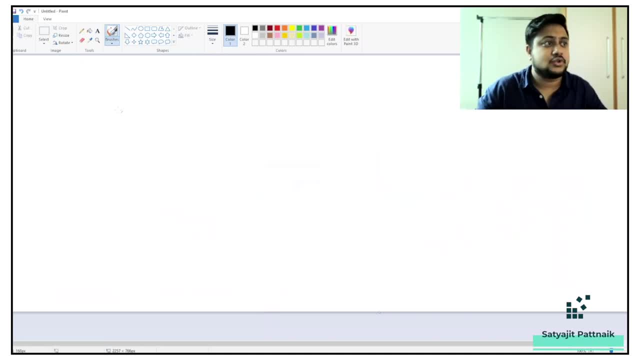 That means the data is. you know, we don't have very good predictors, but still This is nothing but a correlation matrix. Like what is correlation matrix? Everybody should be aware of it. That correlation is always within the range of minus one to one. 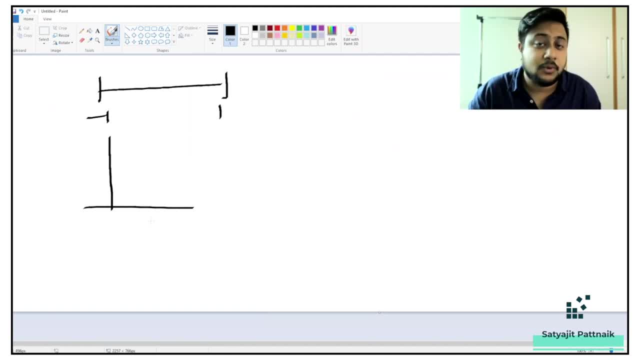 Where? what is correlation? Let's say I have two columns, numerical columns: height and weight. If your correlation value is near to one- 0.8, 0.6, that means height and weight are positively correlated. That means if height increases, weight is also increasing. 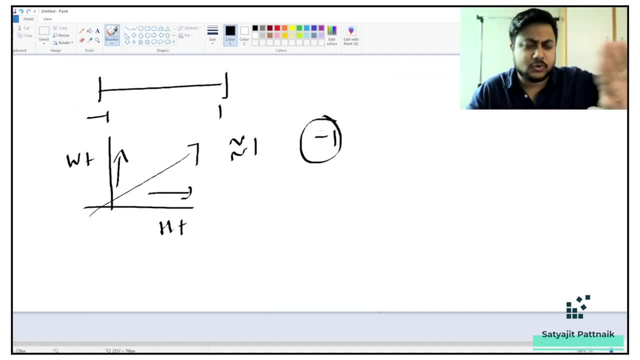 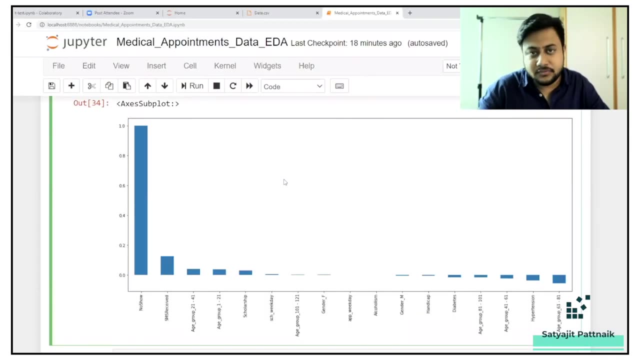 If the value is near to minus one or towards minus one, then it is negatively correlated. That means if one variable increases, the other variable decreases. Any number near to zero means there is no correlation. That means both the columns are independent of each other. 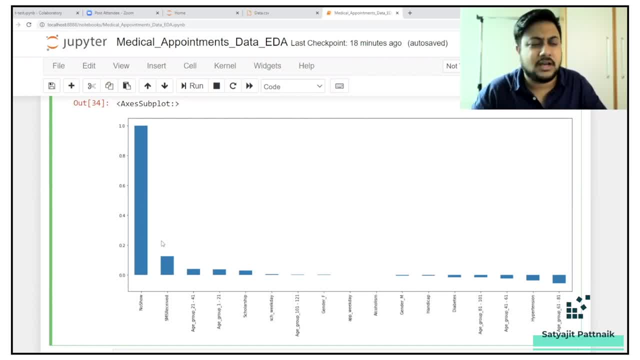 Of course, this value is not very high, but you can just assume it to be highly correlated because, as comparing with the other columns, this is how one of the best predictors can do it. This is how one of the best predictors looks like in this particular use case. 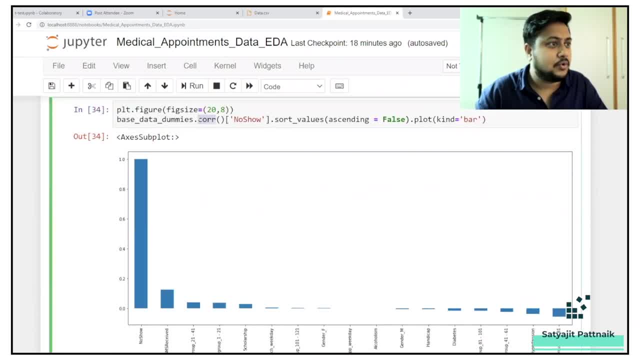 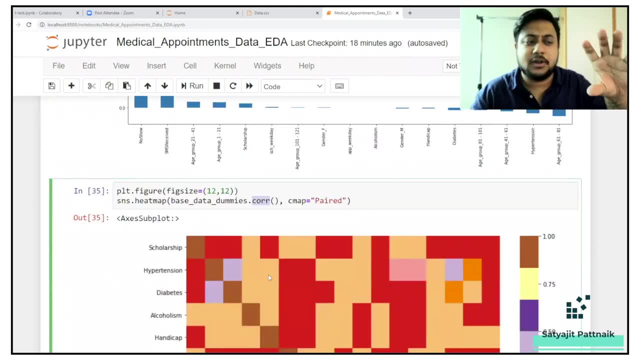 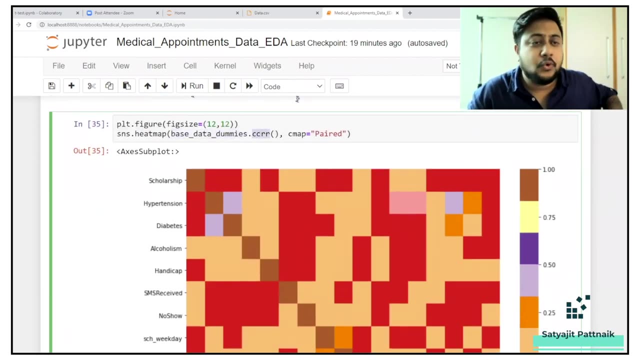 Same thing. I have just plotted a heat map. The same correlation function. I'm just plotting a heat map, You can see. oh, this one is. there is a simple difference between this one and that one. This one, the heat map, is basically a full data frame correlation. 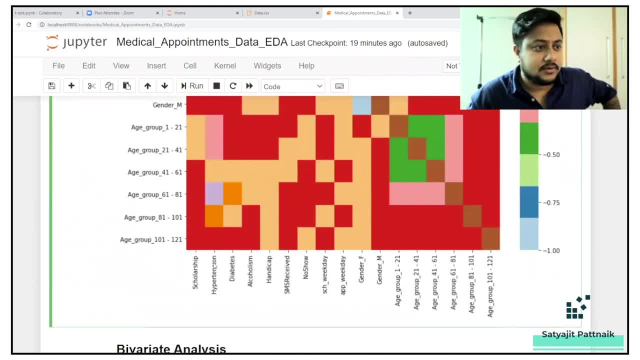 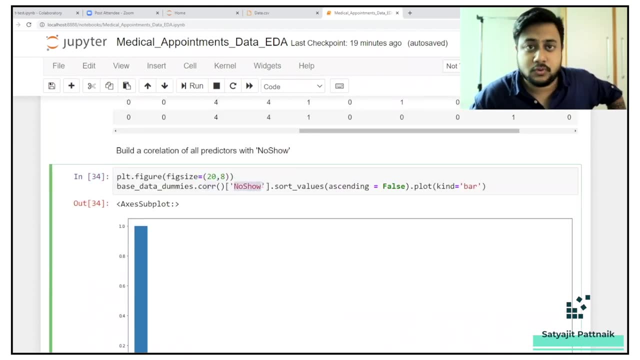 That means each and every column is giving a correlation number with each other. Let's say, age Group 41 to 61 with respect to scholarship is somewhere around 0.0.. And this one is correlation with respect to no-show. That means our target variable. 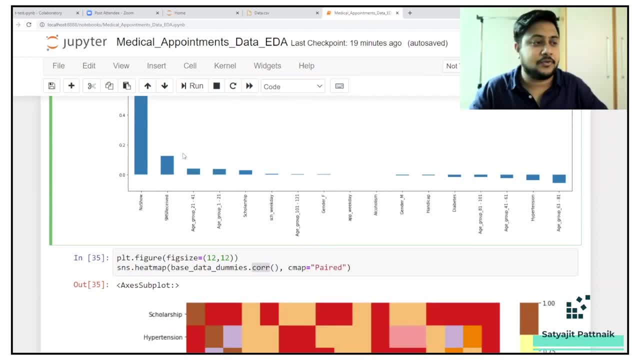 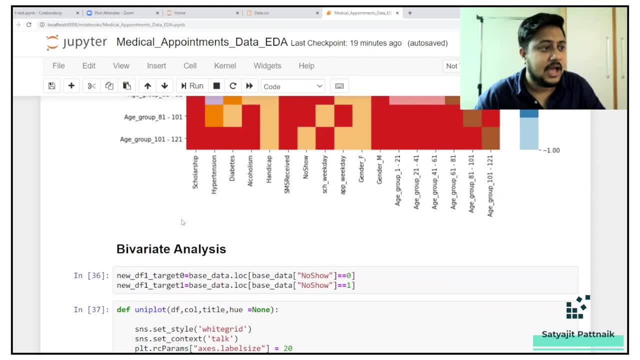 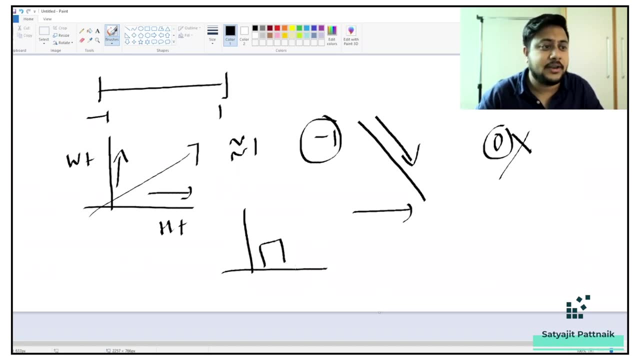 So SMS received is highly correlated towards our target variable. Now, after our numerical analysis is done, then comes your categorical analysis. I hope everybody knows about bivariate, univariate and all those things. Univariate is simple, It's nothing. but you are analyzing one. 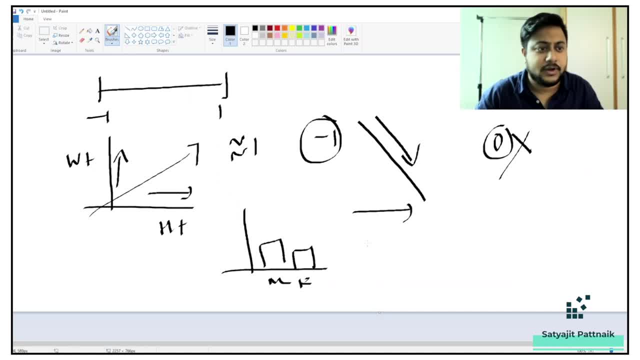 You are analyzing the column. That means male is to female. What is the ratio of male is to female on the original data? Let's say 50-50.. What is the male and female ratio for the no-show data or the minority class? 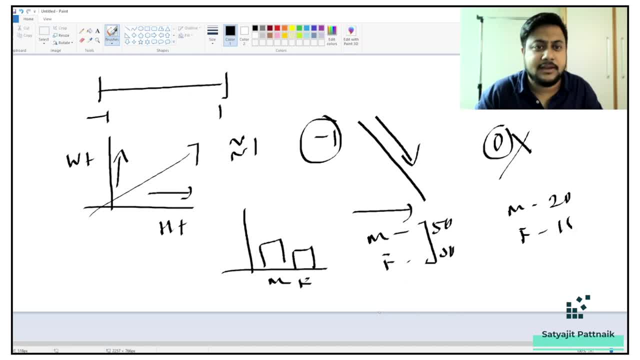 So let's say 20 people and here 18 people. So somewhere nearby, right, If you see, males are 100, females are 20.. That means males are higher in number. So these are the intuitions which you can get. 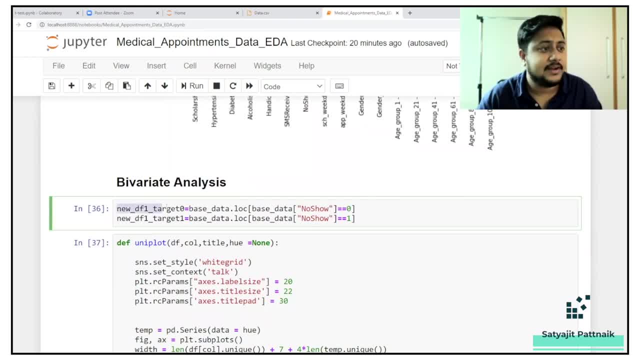 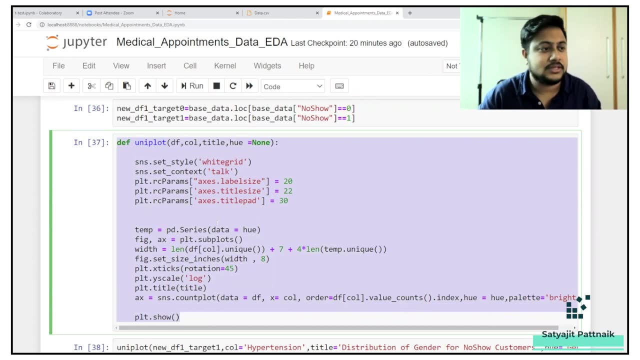 And next comes your bivariate analysis, where I have created two different data frames And here, for no-show 0,, I have target 0. for no-show 1,, I have target 1.. And then I have created a small plot. You can directly copy paste this code. to be very honest, don't go through this code line. 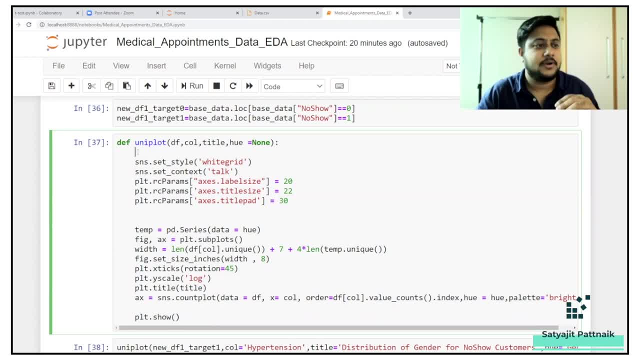 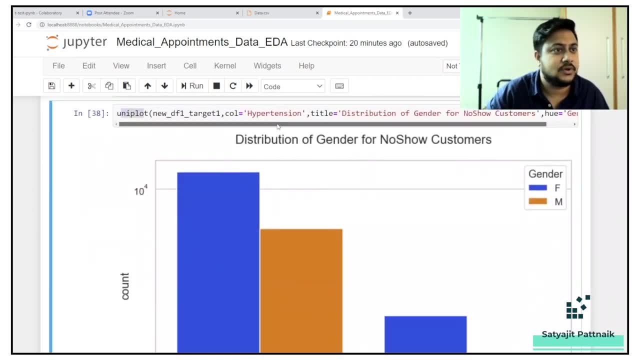 by line might be a little bit complex for beginners, but you are free to understand it, Okay. Okay, So I have created the same plot and I'm getting all the distributions You can see: hypertension with respect to gender. So what is the intuition here? 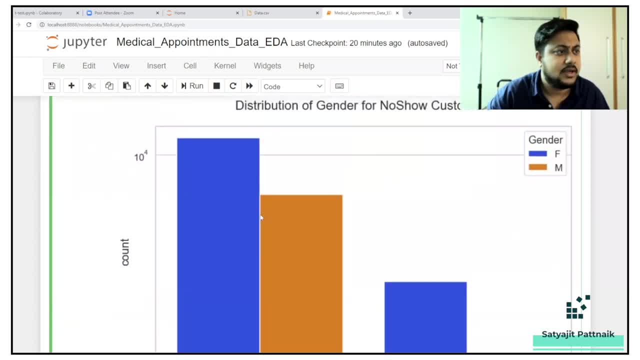 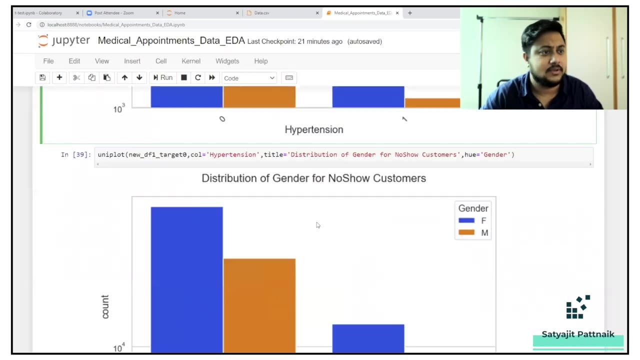 Hypertension with respect to gender for target 1.. So it's like for 0 hypertension you can say almost 1000 records are there with for males and females, like males are higher in number. So this is the intuition which you can get from different graphs. 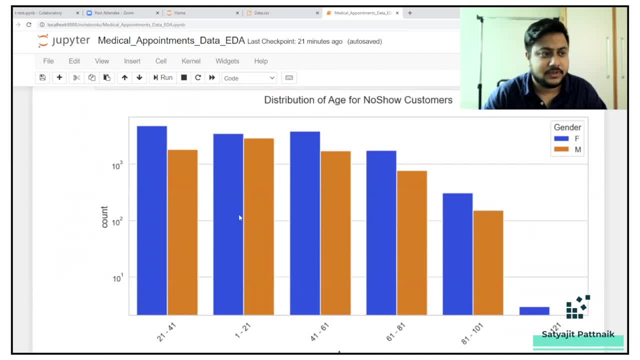 Okay, And then you have to analyze each one of them, like for this particular age group. and this particular age group you can see here for 101 to 121. So I don't see any males here. So all the records are female records. here for 1 to 21, I can see almost an equal ratio. 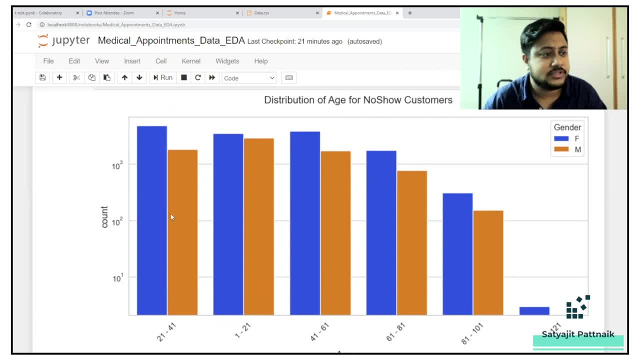 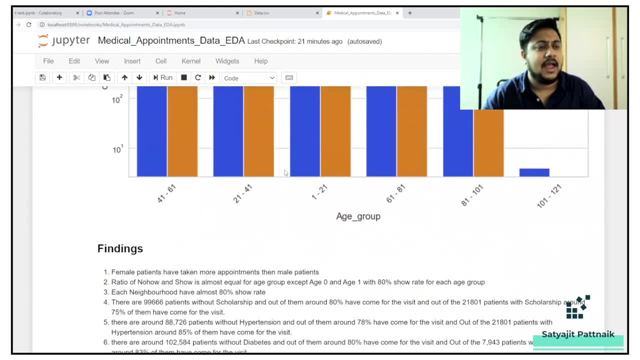 of male and female, but with 41 to 61 or 21 to 61, females are more in numbers, Right? So this, this, these are the normal intuitions with you, Okay, the? that's the task of a data analyst and a business analyst. data analyst uses the different. 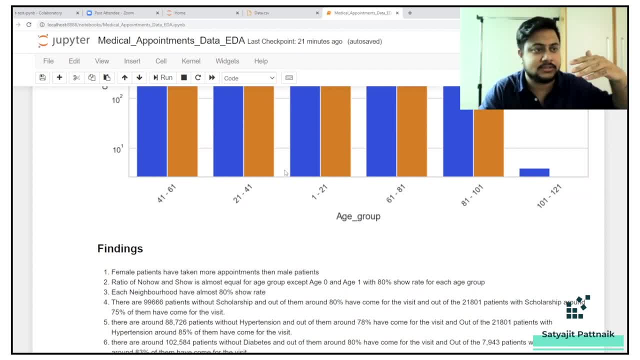 statistical analysis, categorical analysis, numerical analysis, all these things to find intuitions, and business analyst basically takes the insights and try to create some presentations or some sort of data visualization, dashboards or reports, something like that, so that it can be presented in front of your higher management. so that's it. you can see the findings here. female patients. 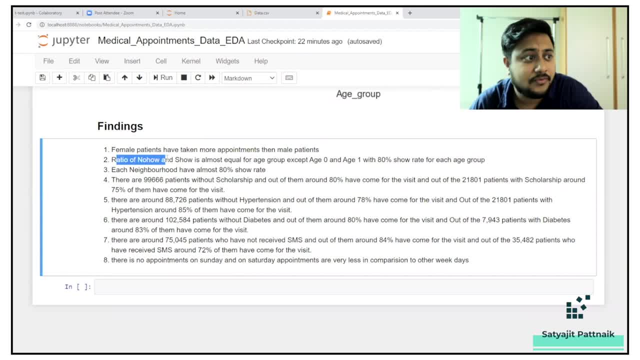 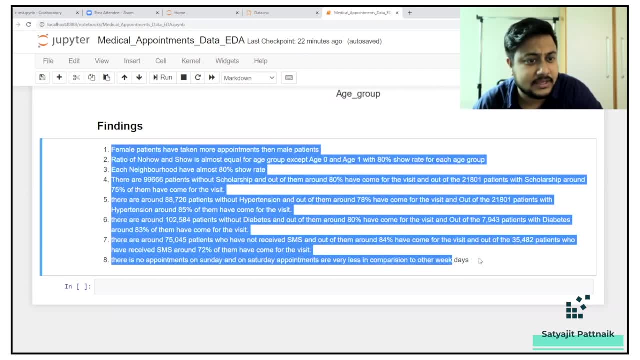 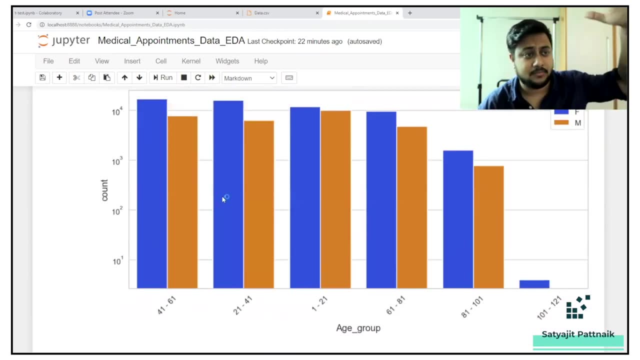 have taken more appointments than male patients. ratio of no show and show is almost equal for age group, except age zero and age one. so you can see, all these are our findings. i'm not sure if we can drastically see some good insights, but this is how it is, the methods, the way of dealing with the eda. 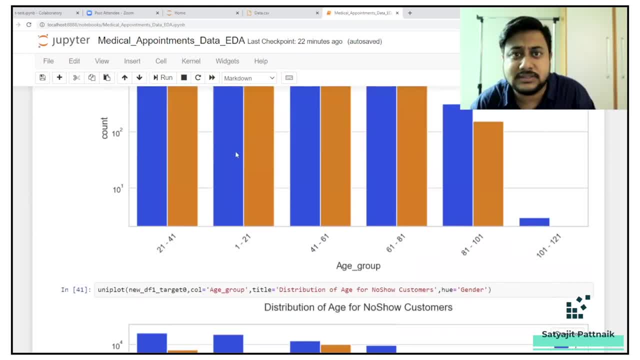 has to be like this. so that's it from today's video. guys, i hope you learned something. in case you are not able to understand a lot about it, you definitely, definitely. the recommendation is that go through my end-to-end eda playlist, like the eda video, which is around two hours. you will get a lot of information from that. 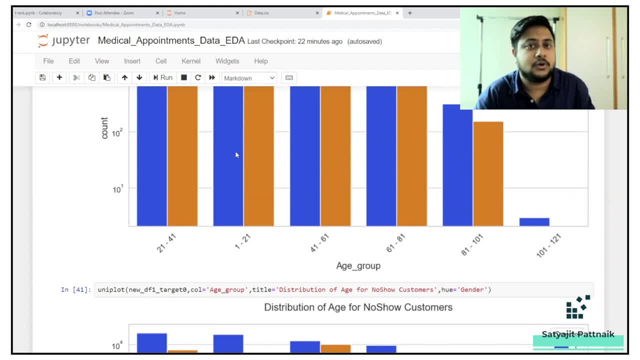 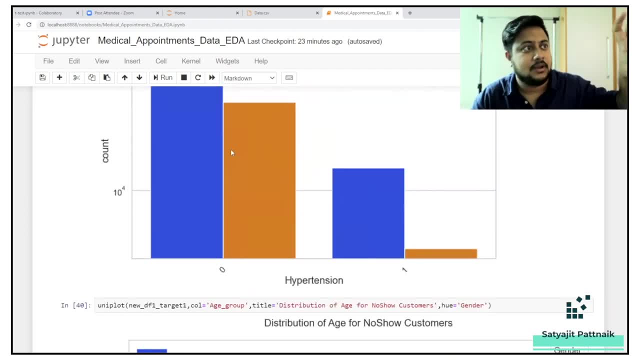 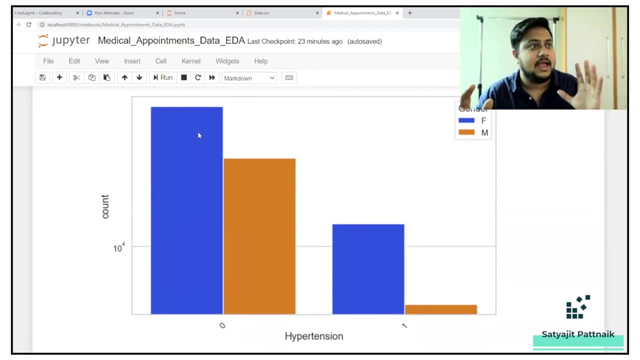 and i'm trying to keep this video short because i don't want to do another two hours of video. so this video is very specific to the healthcare part and i will leave this data and the file, all these things, in the description below so that you can run it and do your analysis. and this is a go. 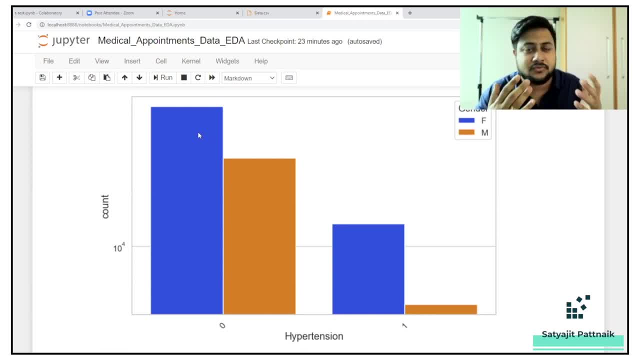 to tool or a go-to code for resumes. if you are fresher, you can definitely add this in your resumes as well. okay, that's it from my side. guys, i will come up with a lot of power bi stuff. tableau is something which i'm targeting as well, but my immediate target is to finish the statistics. 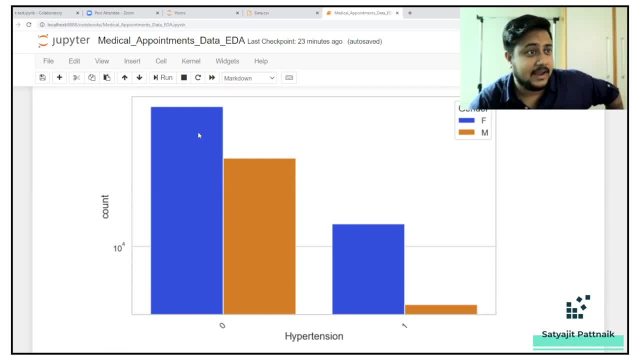 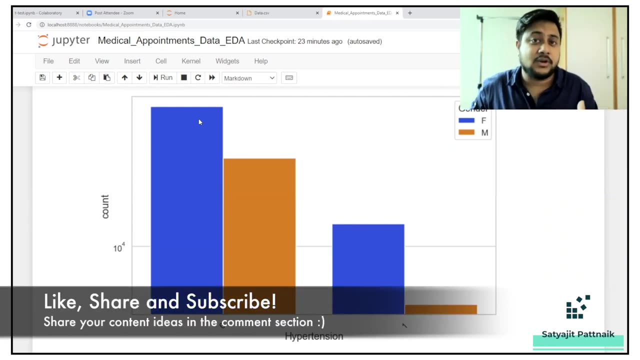 part and the eda and power bi part. that's it from my, my side, guys, thank you. if you like the video, please like, share and subscribe. if you want any sort of videos related to this, for example, if you are coming from a mechanical backgrounds or from other areas, let's say you want something into. 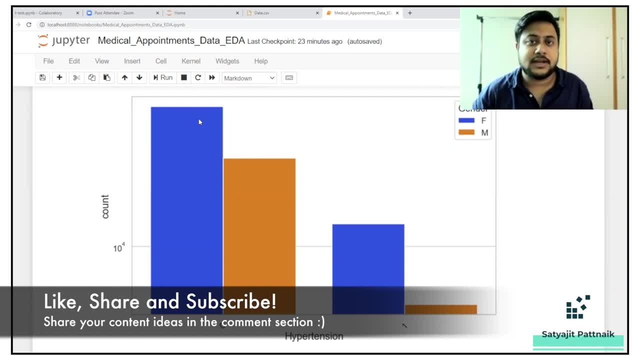 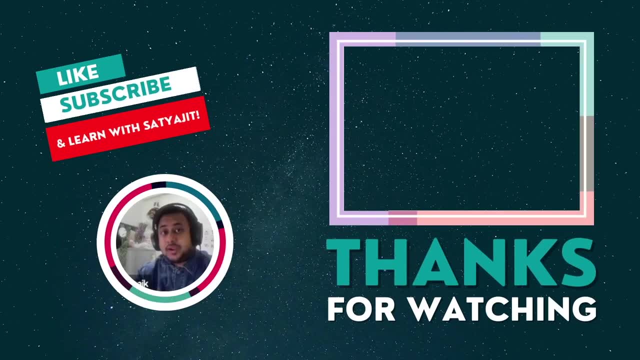 banking or insurance. let me know in the comment section below so that i can create a video for that as well. thank you guys, bye, bye you.